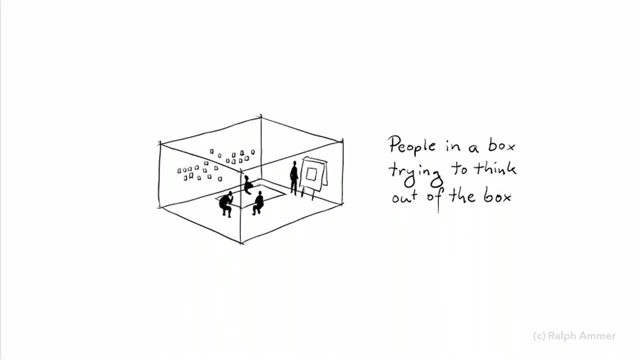 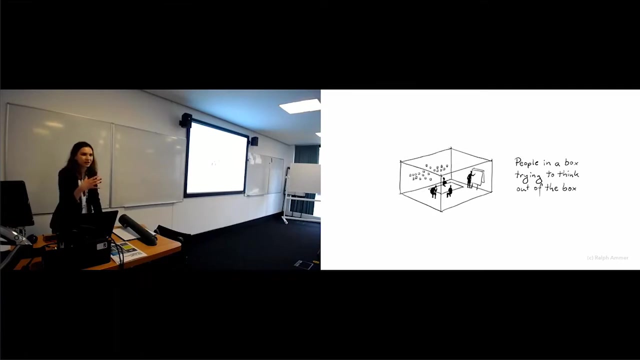 methods. I know that the next week is the week of self-reflection for you, where you need to come up with your own ideas, project ideas, and try to go out somewhere, walk around the park and think about this, but don't stay in your room. 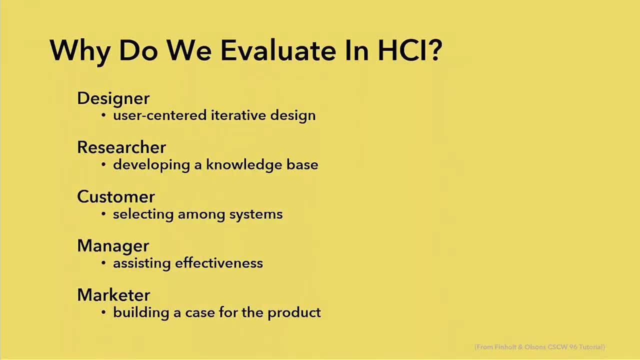 So why it's important to evaluate human-computer interaction from the multiple perspectives. So we have the designers, researchers, customers, managers, we have users. we have different agents who are interested in the final product And from each perspective it's important. 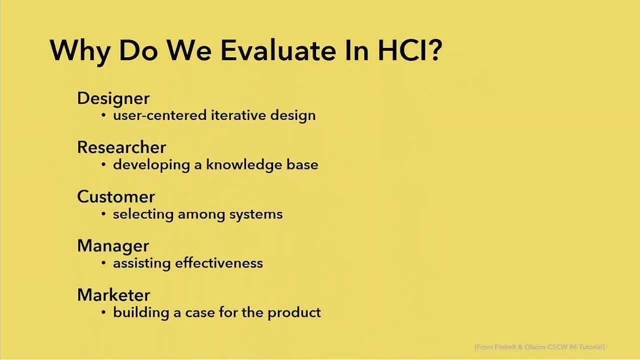 to qualify the standard of the product and make sure it's good. Thank you, So it's the best. Designers are interested in the user actually. So the person is the human is the central part of the whole hierarchy of the life. Researchers like myself, we are interested in creating. 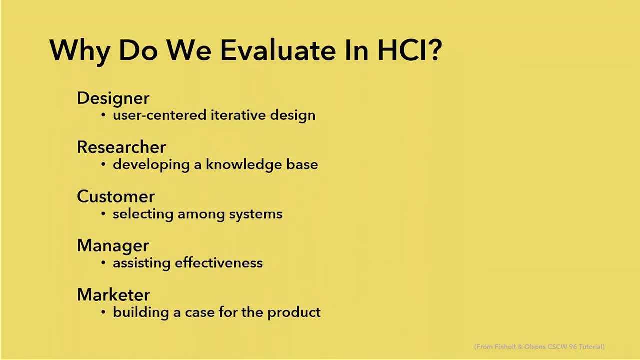 the knowledge base. We're interested in inventing new methods, testing existing methods, understanding what's not covered. what's things that they're looking for, Managers? well, not really. They try to guarantee effectiveness of the system, of the tools that they're using. 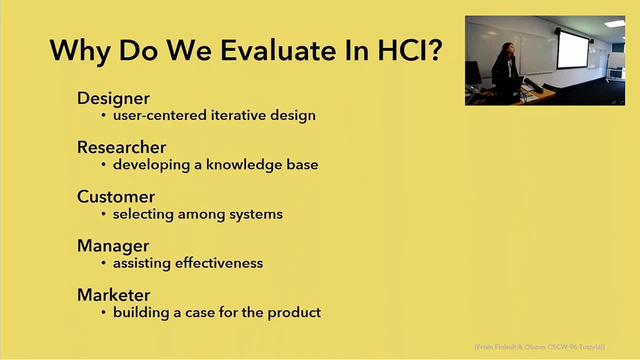 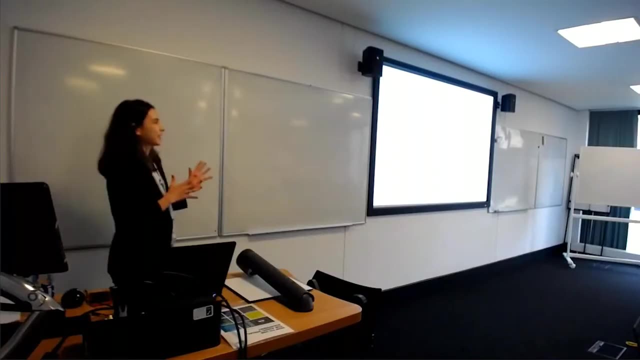 And finally, marketing team wants to showcase something to guarantee the nice performance of their unit or the company. This is how it works, the whole interaction. It's a very super mega-complicated scheme, but actually it's very simple if you look at it from the perspective. 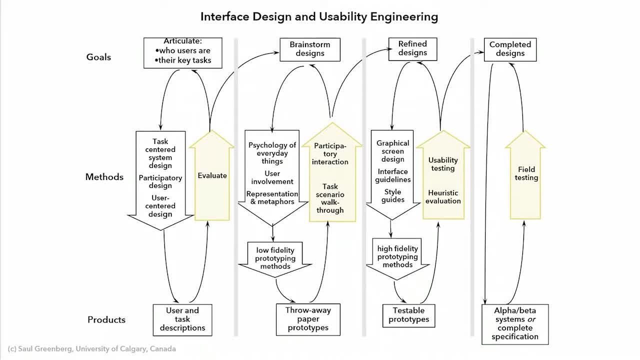 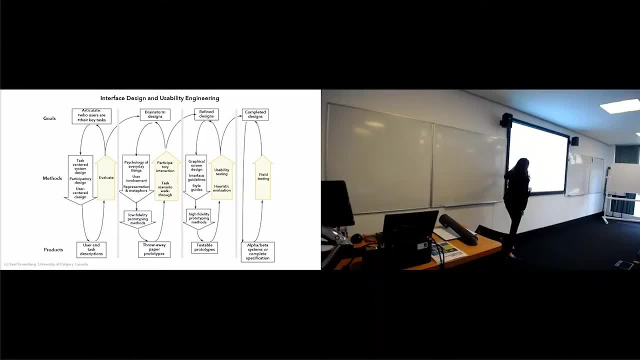 Okay, Yeah, so this is like a cycle of how people evaluate things. At the top, we have goals like: what are the goals on each cycle of the user interface evaluation and usability engineering? In the middle are the methods that we're using, so we're constantly changing our methods based. 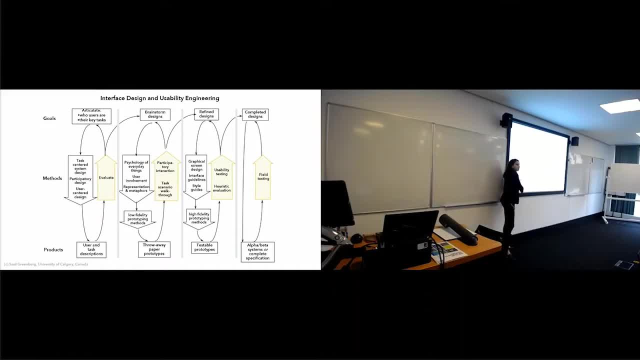 on our face. And the last is the products that you're supposed to have at the end of each cycle. Okay, So the first one. They don't really have a name, It's like a face one, two, three and four. 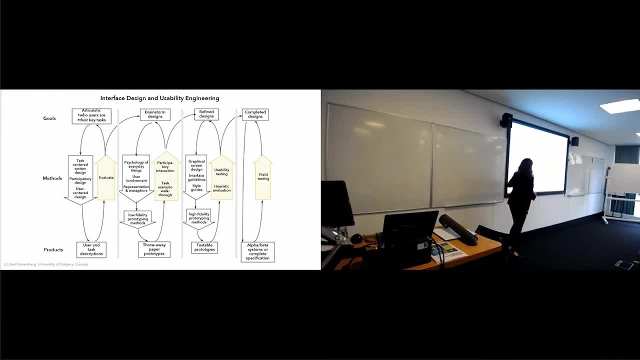 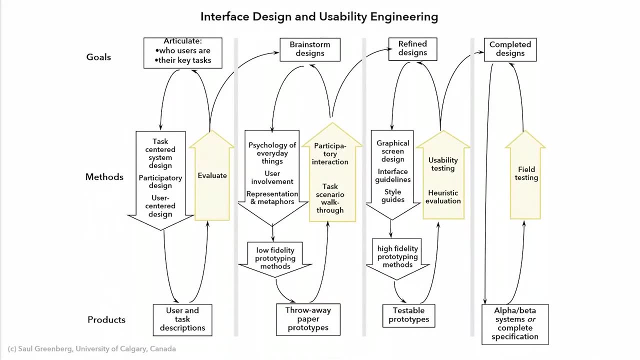 It depends on the product that you're working on, that you're building. You might want to skip the face if it's something really simple, But the goals actually are quite identified for each case. So you try to understand who your users are. key task of the user: what user is performing? 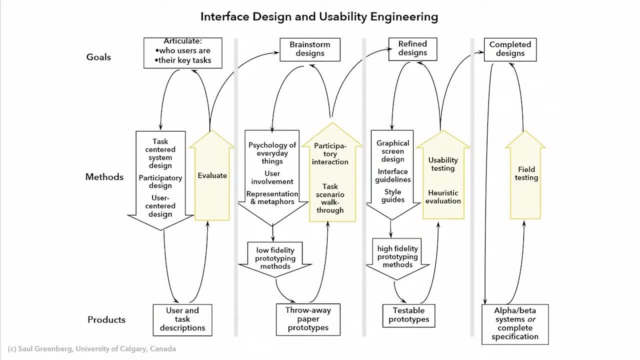 during the first phrase. Then you need to understand the designs. So designs of your product: Okay, Is it a mocap? Is it like 5,000 images of something? Is it a new holographic car or something else? Then you basically repeat. 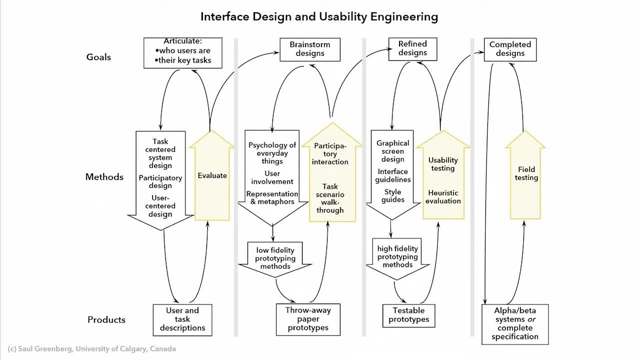 You redefine your design, You correct mistakes, You get more data from your methods that you gathered, for example, from the interviews or different discussions with the user, And, at the end, your goal is to complete your design, to finalize your design and have the 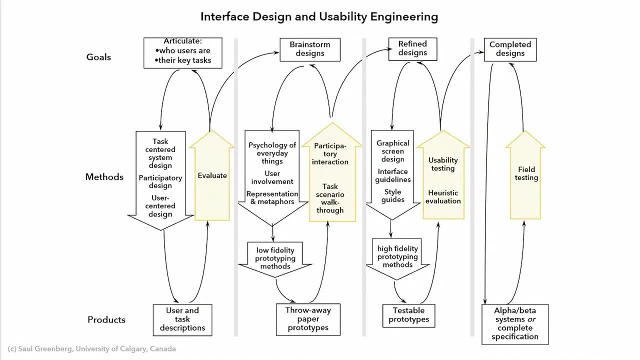 final product. Okay, So the methods are, as I mentioned before, are different during each phrase of this cycle. They're all user-oriented because we just want to talk to users. This is human-computer interaction. We are first of all evaluating our human because we want to understand our users. 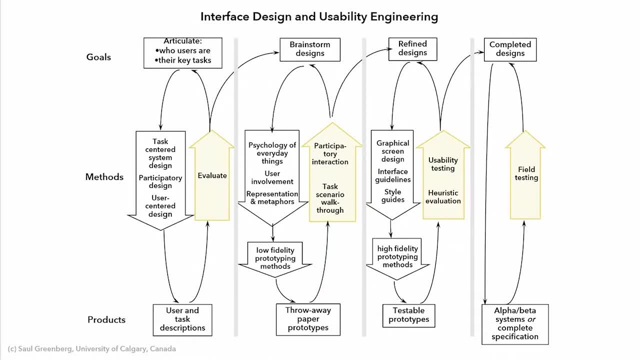 And at the end we're evaluating our system. So the task-centered system design, participatory design and user-centered design are three methods. These are the methods that are used during the first phrase. These, basically, are the designs methods that are trying to understand who are our users. 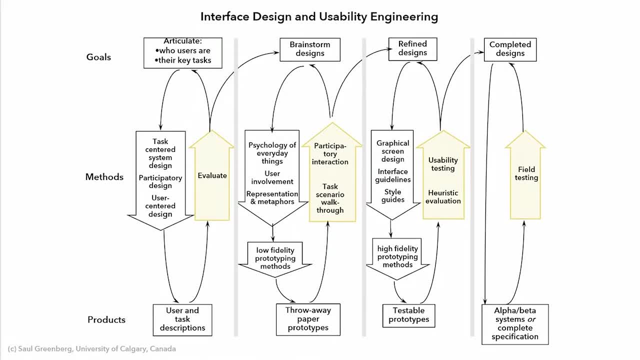 and what they want to do: interview techniques, different conversations and discussions. I will talk about the methods within them later on, But these are mainly those methods understanding the user. Then we create our first product. It's a user task description. It's about who they are, their age, their education, profession, preferences, hobbies. 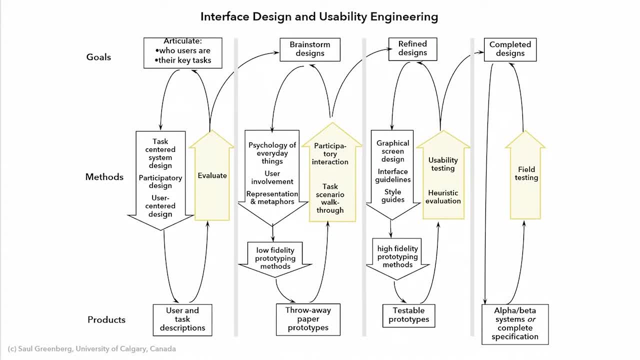 et cetera, et cetera, all this, all the data that you can gather from the user. Then we evaluate that and you create new designs. So, for example, you need to create a new system where people can choose the presents for their 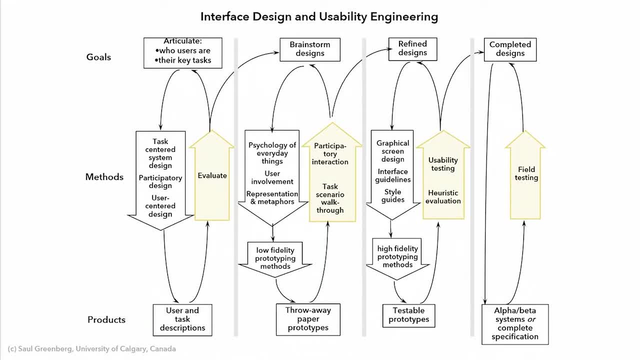 family. So it's like augmented reality shop where you can buy anything. The second phrase is to create low-fidelity prototype. It's basically the same thing. It's the same thing. It's basically the prototype that you create from secondhand things that you have at home. 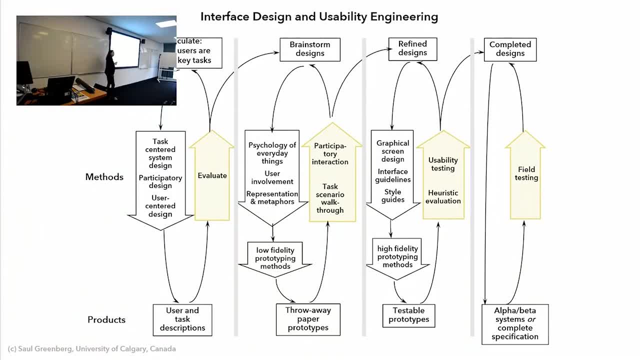 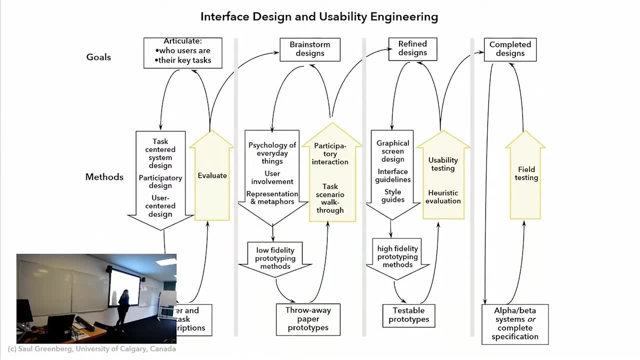 from paper, from rubber bands, plastic strings. It's something that like hands-on and really easy to do at home as well. Then, finally, you've reached your goal. You completed your design, and you're stuck in this constant loop between field testing and your complete specification prototype. 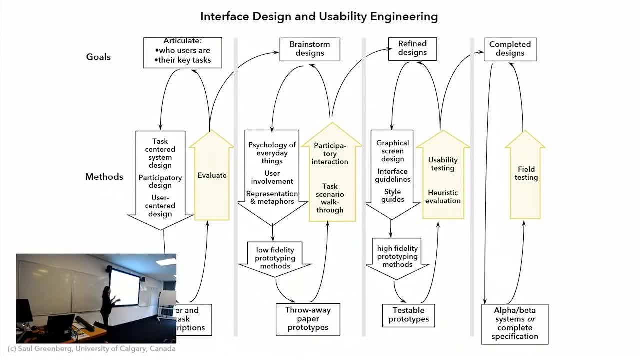 Great, Great. Thank you very much. Thank you very much. Thank you, It was a pleasure. You have this like car. You 3D printed your car or something else and you go to the user test it, go back and 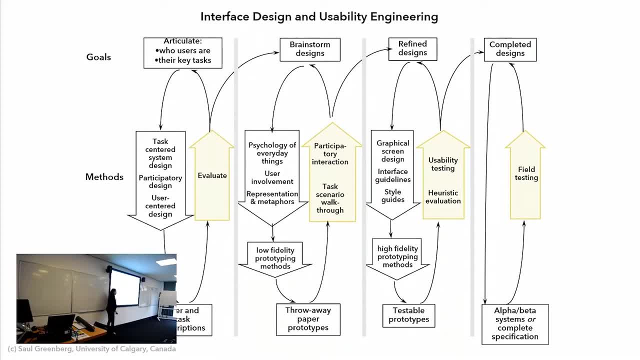 release the new version of the prototype. Usually this process can be modified. It depends on your needs. You can have different methods in the middle, but you may notice that it repeats itself. the feedback, because you always get a new impressions and a new ideas of how. 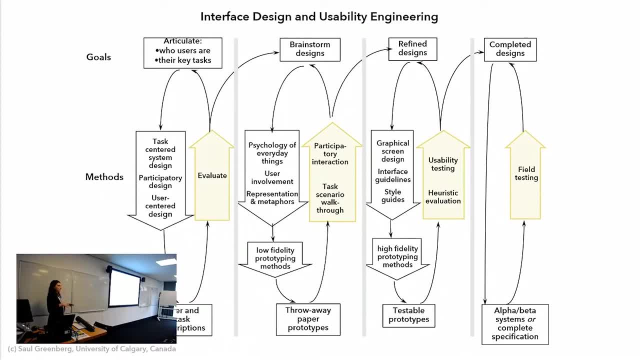 that how the product needs to be changed. sometimes it's not wise to listen to the user because the user might not know what she, she or she wants. so it's always need to try to be critical and think critically about the, you know, normal ages, ages of common sense, and try to trust, first of all, your aims of your. 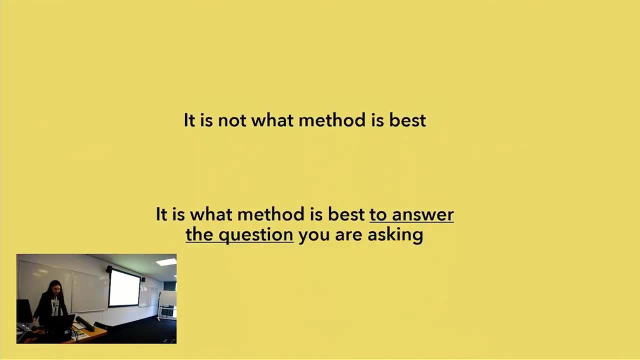 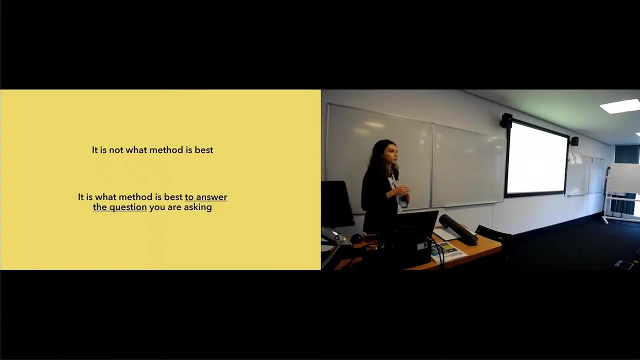 project. so yeah, maybe the logical question is like: what method is the best? and it's not. what method is the best. there is no like this is the best method. it's always the best method that answers your and your question that you're asking. sometimes one method is absolutely perfect for one reason, but 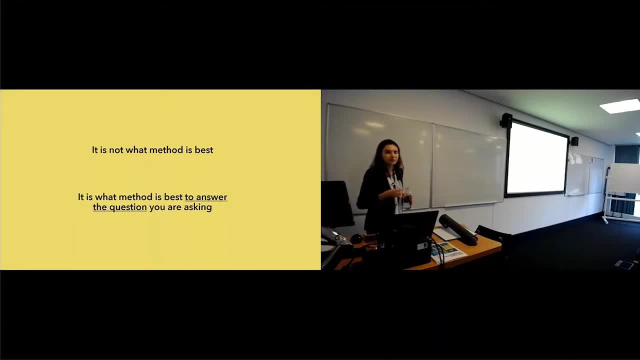 when you're working on a similar project but your aim and research question is absolutely different. it's just better to use a different method because it doesn't have any qualifications to fulfill that goals. and why do we need to use different methods? because, well, it's, all methods are different and they fulfill. 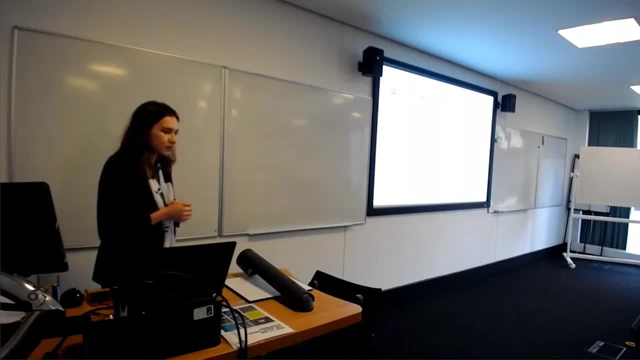 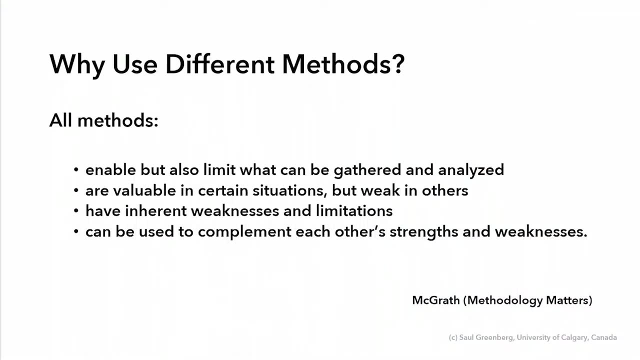 different needs. for example, during the this spatial computing era, I personally was trying to understand how to evaluate spatial interface and how to evaluate spatial systems so we can use spatial systems to evaluate spatial systems. so there are not no existing methods evaluating augmented reality interactions in augmented reality user interfaces. I tried to revisit all the 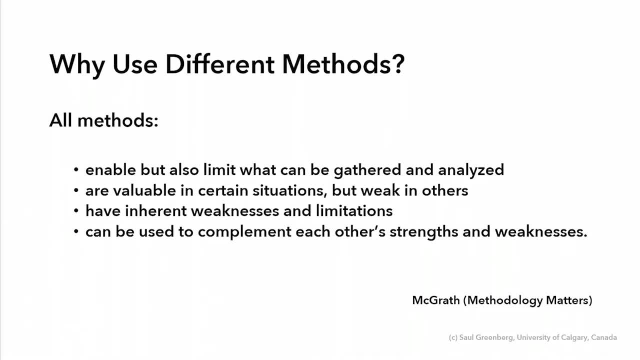 existing methods, all the existing usability methods, and I understand that they just don't cover the aspects such as navigation in the space, personal interactions with the physical environment around in the room or in the different spaces, and in this case we, in the lab, we created the new. 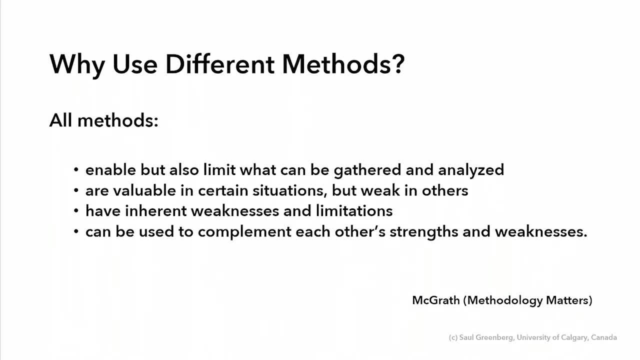 model and we created the new model. and we created the new model and we created the methods to evaluate spatial user interface design. and sometimes you need to mix your methods because they're more valuable. for example, you want to mix interviews and some a quantitative test. each model has its own weaknesses and 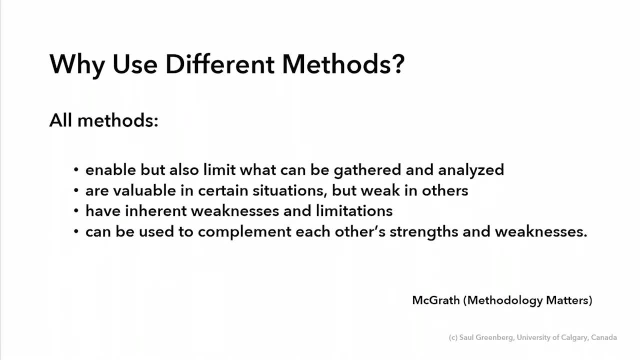 limitations. if you read upon one method, you might want to say, okay, it has its own weaknesses. and in this case you think, okay, I will fulfill this by doing another method, but it's not going to be the same method that I'm going to use by doing some interviews and something else. and also it's a common in research. 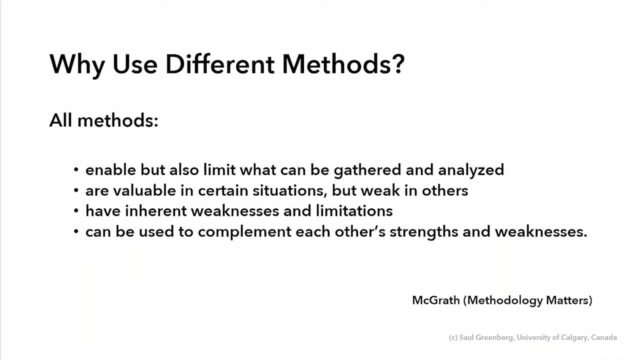 when one method complements another and giving more data to analyze, giving more data and more insights to support your hypothesis or a research question. it's all relative as well to the non research aims, when you're trying to find how the product will behave in a different environment, for example. so 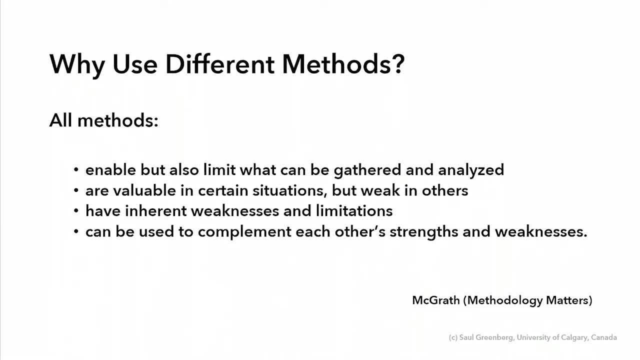 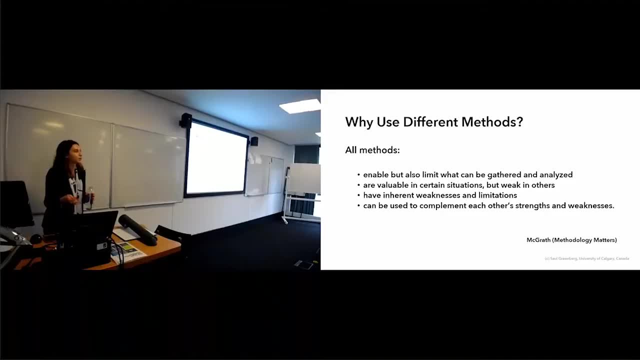 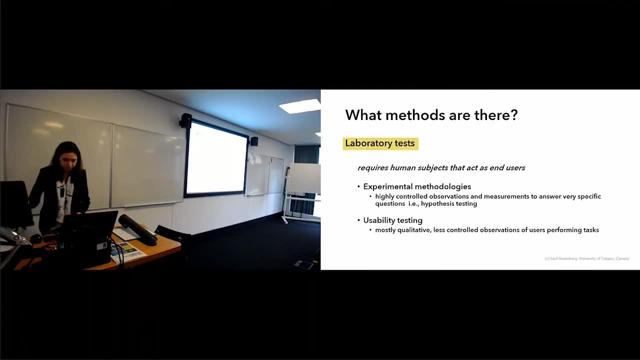 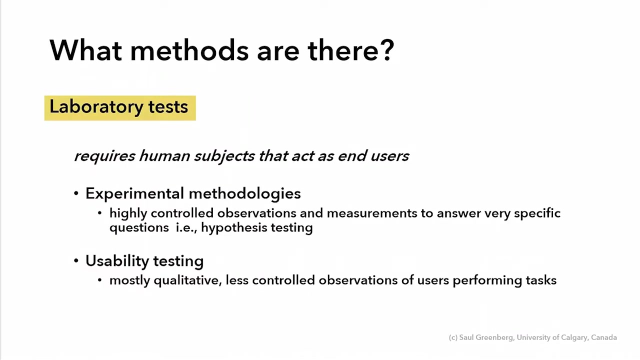 this time, when we looked into it, it was more the non research one, which is allow the user to work from an actual perspective, and it would be moresighted. so you tried to always find which of them helps you to get the data that you want from the user. 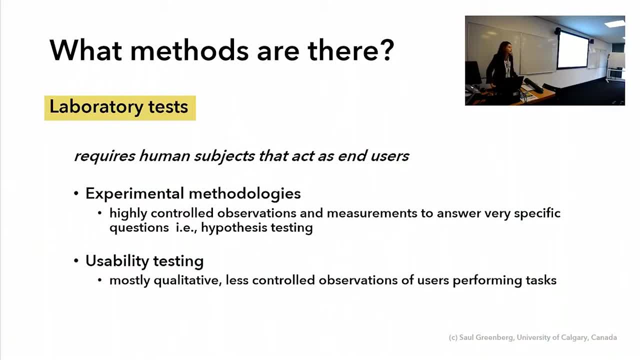 And for that you need human subjects actually to be in the lab. So these are the highly controlled observations. when you're looking at the behavior of the people, It might be something like you gave a prototype to a person who is sitting in the room and then you're observing that person from this mirror glass wall, like in the police department somewhere. 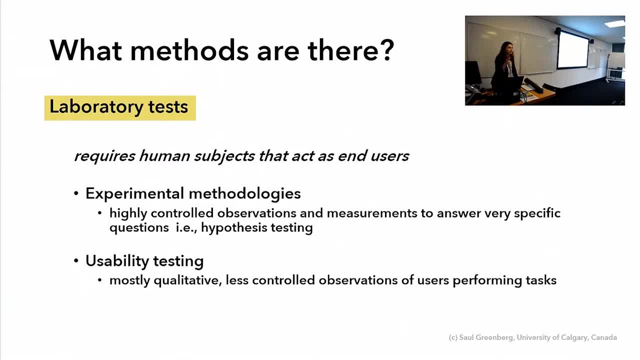 So you're trying to understand how that person reacts and behaves And that is a highly controlled environment where you want to correctly and really precisely answer your question, your hypothesis And some usability testing in the lab. So there are less controlled observations, but you're giving persons to try your prototype and you observe the behavior. 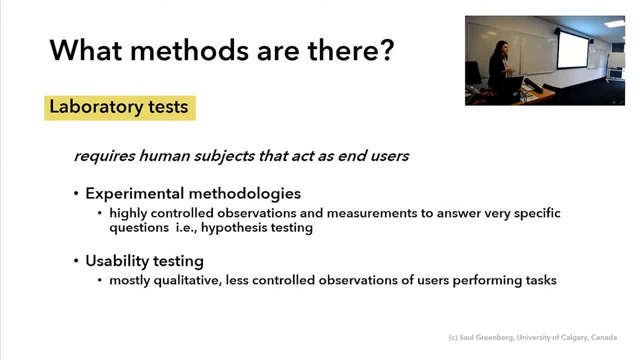 It's basically descriptive methods where you describe how the person behaves. It's like if you created the AR application and you want to see how the person will behave in one particular environment. That's the method you will use the usability testing in the room on site, for example. 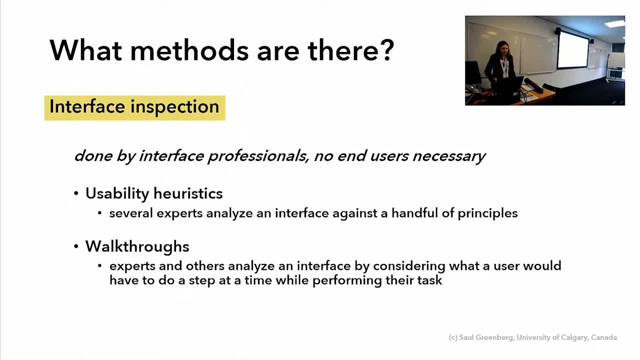 The next one is interface inspection. It's basically. you don't really need to have real end users with you at the end. You can ask your lab colleagues or someone who is specialized in user interface. You can ask them to do the evaluation. 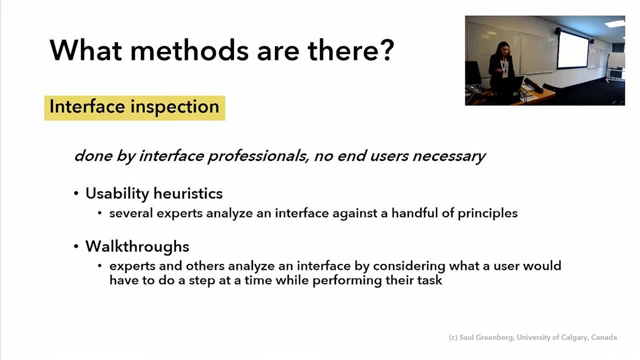 It's called usability heuristics. Where several experts analyze Heuristics are the statements It's like, for example, a statement of: I can see the progress of the application is visible. Do you know that the progress bar, for example, when you're loading an application? 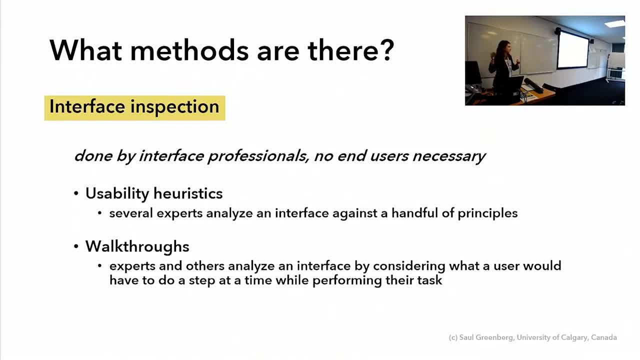 you see the progress bar and you can track how long does it take to finish that. And heuristics are the statement. The collection is the statement, The collection of the statements that researchers collected to describe particular things. There are three main groups of heuristics. 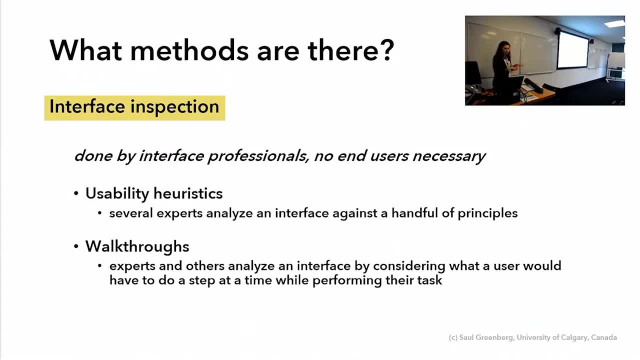 The most famous is Norman's group of heuristics. I didn't put it here because it's really a deep topic, But basically it's just a classical set of statements that you want to apply to the product, to the application, when you're analyzing something. 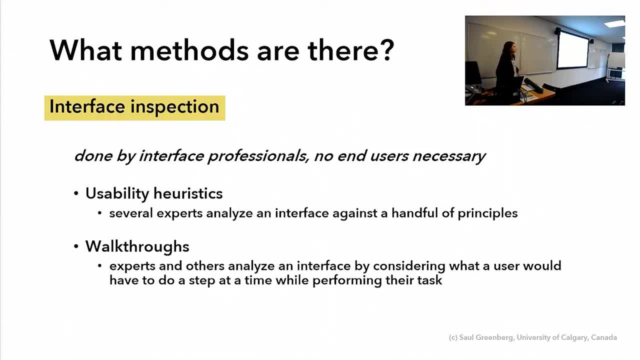 And statements are like. I was able to see the progress, I understand my state, where I am now in the system, et cetera, et cetera, And also the walkthroughs. It's where the experts analyze, analyzing the interface. 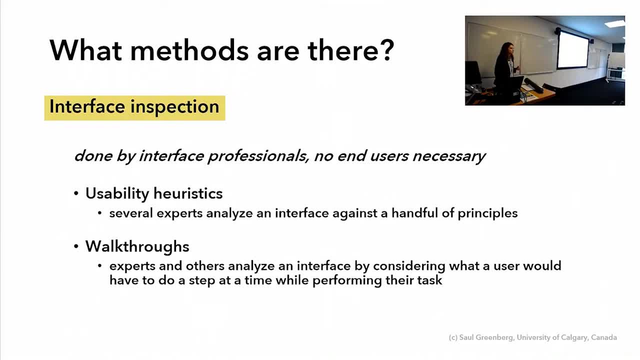 when someone is performing the task. So classical example with AR someone is wearing the HoloLens And basically that person is talking while doing what he or she is experiencing right now And the researcher or observer can ask some additional questions And the conversation is recorded or video recorded as well. 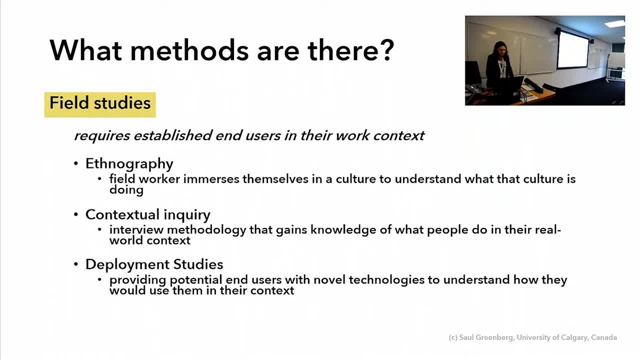 The next method is field studies. It's not so. I wouldn't say that it's fairly relative to augmented reality, But it's a classical method for sociology, And since HCI is some part of sociology as well. But it's basically the step where you will immerse yourself. 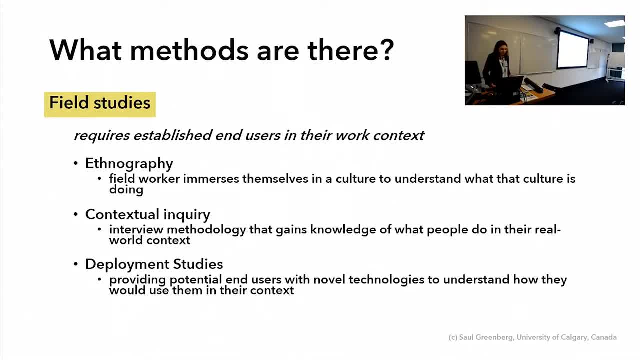 Into the environment of the user. Ethnography is the classical example. You try to understand the culture and the behavior of the person. So, for example, you need to create an application for a hospital. You've never been there. You have a brief understanding of how it works, how it looks. 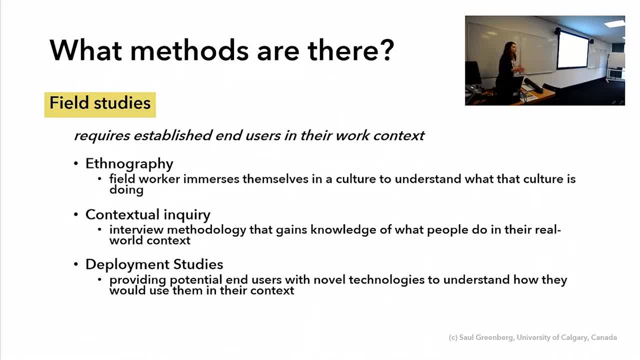 But you need to understand the system, for example, of an IRI EMR unit, emergency unit anyway, And you go there. You spend a day a week, three weeks, depends on your needs, And you observe everything that you see. 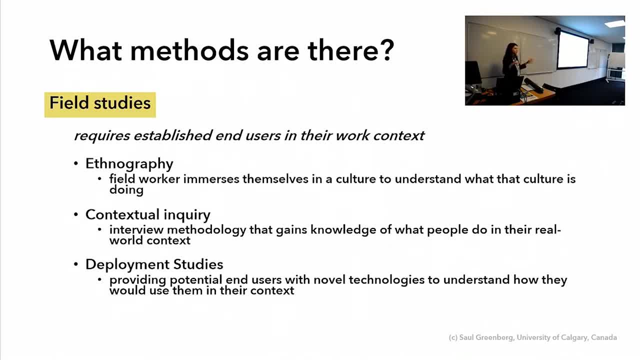 You don't really need to ask questions, You don't need to interact. The important point is just to be really attentive to all the things that are happening in the environment Or, for example, in the classroom. you see how people, for example, walk around something. 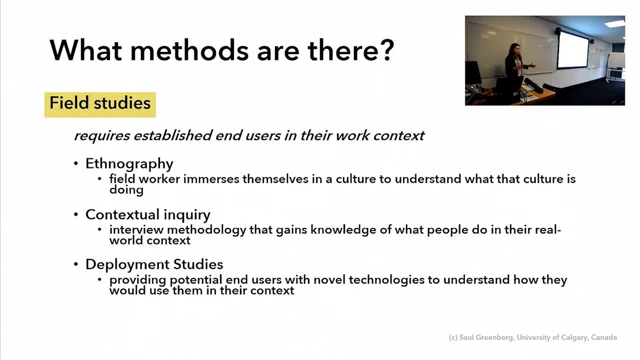 Maybe the path that they're walking is not really comfortable And you can spot that. OK, I can change this by doing A, B and C, So it's really about observing These two below- contextual inquiry and deployment studies, are similar. 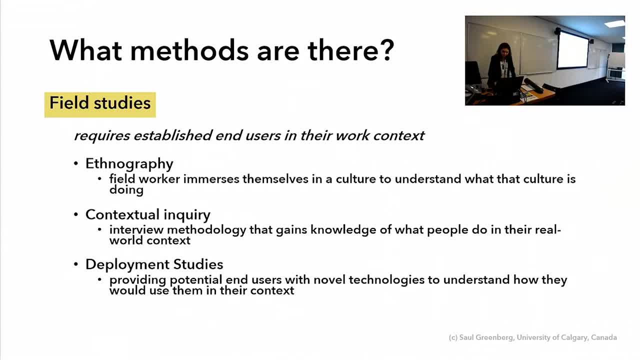 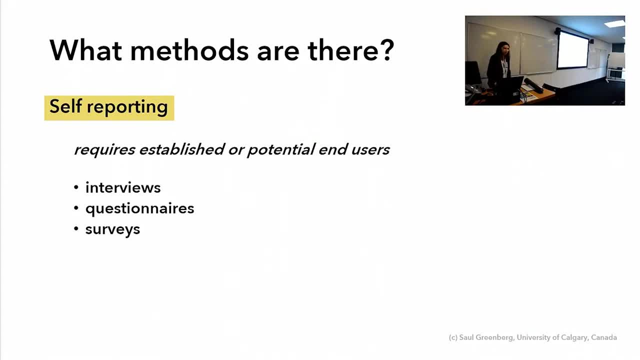 But ethnography is the most common where you immerse yourself. The next one is self-reporting. This is a very super classical and the most used methods: Interviews, questionnaires and surveys. Questionnaires and surveys are really easy to conduct because you can just simply send a link and collect the data that you will analyze. 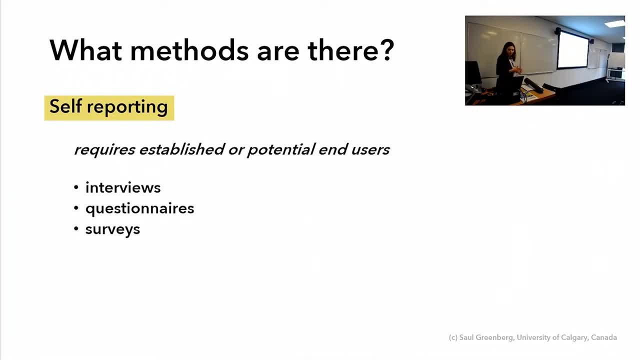 It's the standard quantitative methods Interviews. there are many types of interviews: Structured interviews, semi-structured interviews, unstructured interviews- It's like when you don't have a prepared script for an interview, for example- But this is the typical methods for people using journalism HCI. 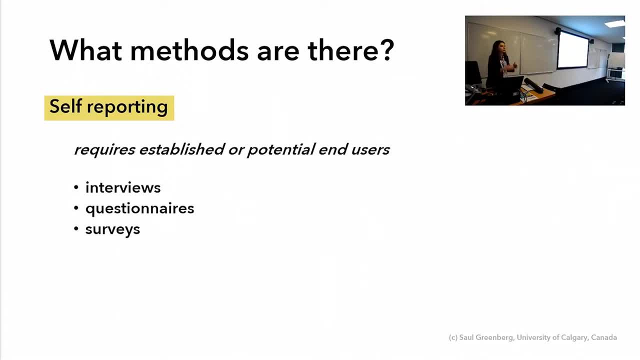 when they need to get an insight from the person And they prepare a list of questions for that. But self-reporting can be biased as well, because it's not an observation. Sometimes people can lie in their questions. You may say: OK, I did that a couple of times when I was too lazy to complete that online survey, or something like this. 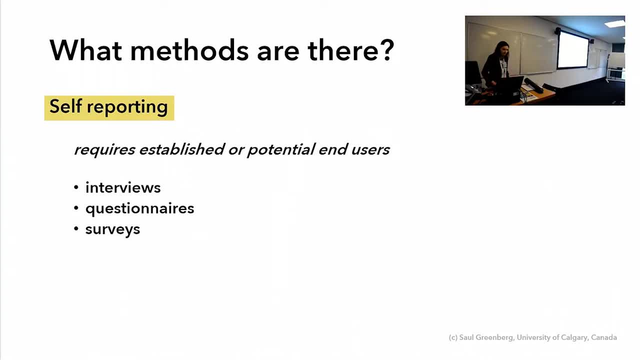 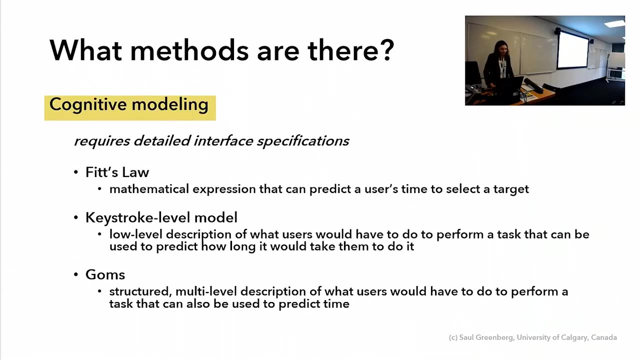 But to collect the approximately relevant data you need to have a big sample. So don't ask one person about your system, Ask 10 or ask 15.. Just have a really nice sample for that. Next way is a cognitive modeling. So cognitive modeling is a method that requires interface specifications. 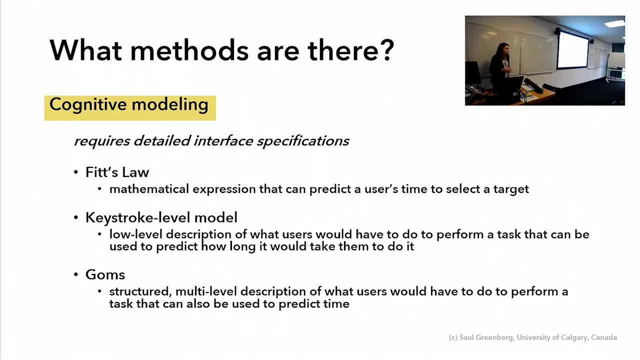 Currently it's used only on the computers, on 2D screens, And these methods are mathematical methods that predict user reactions: Time people will spend on doing something. I will show you a picture in a second. For example, this is the Fitts' law. 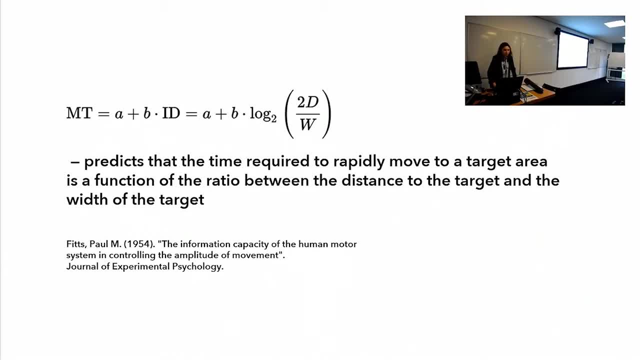 It's like the nice formula And that predicts the time that user needs to spend on moving from one point on the screen to another. For example, how long does it take for you to look from the cross button on the screen to the menu button on the screen? 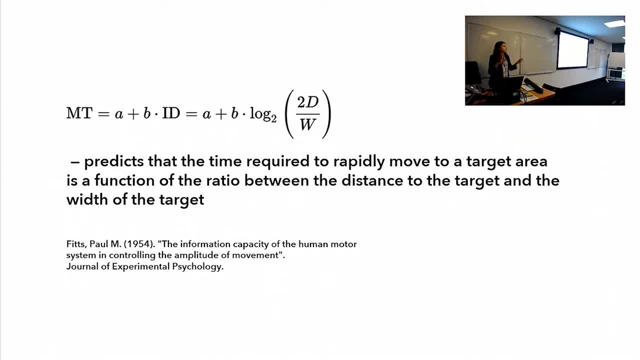 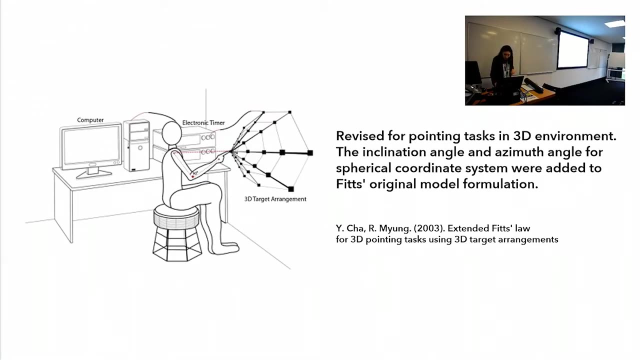 So how people will interact with different parts of your user interface element. And it was really hard to adapt that system for augmented reality because it's really into 3D And there is an adaptation of Fitts' law by Cha and Moing from 2003.. 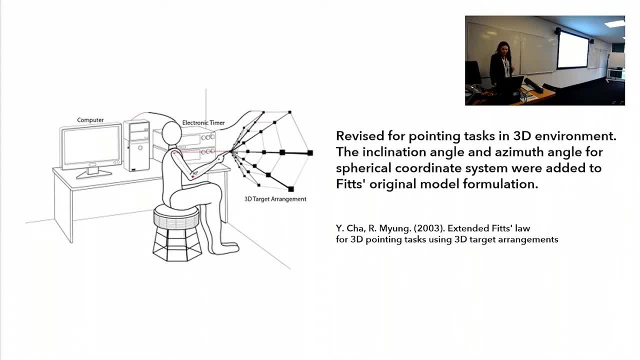 It's like an extension extended Fitts' law. So they revised it and created the 3D sort of timer. So how would you move in 3D? I'm not sure that at this point on your research you will use this method. 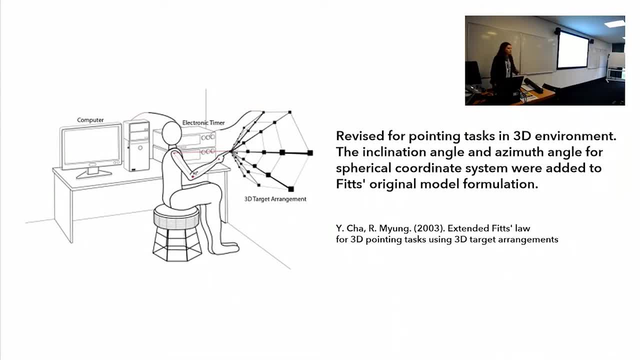 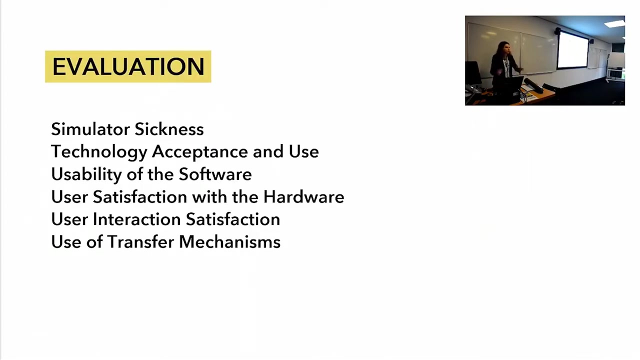 It's maybe something more advanced that you want to use further in your studies or career, But I'm just describing that there is these types of methods And maybe in the future there will be more sophisticated ways of evaluating distances in augmented reality. So this part I just finished with design methods and now it's the research methods. 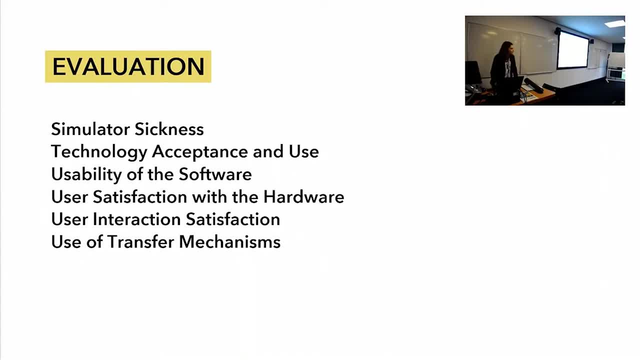 Basically the methods that are mainly self-reporting, quantitative methods that are commonly used, particularly with AR- Because I try to focus this presentation on AR mainly- And these are the methods that we commonly use in the lab during all the trials and experiments- Very common, but you can at some point ask yourself a question. 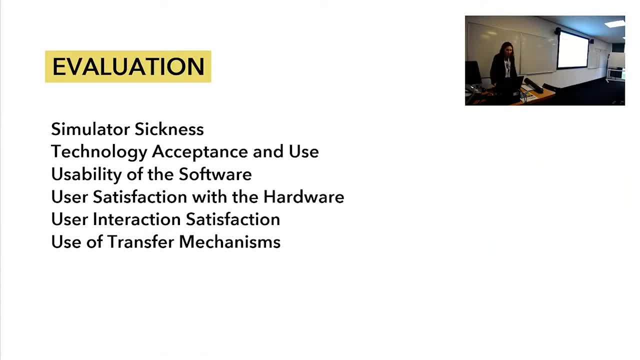 Is it relative to augmented reality? Does it still cover all the needs that you want to have at the end? So the first one is the simulated sickness, So maybe the most relevant to VR and AR, where people are trying to understand whether the system will make you motion sick. 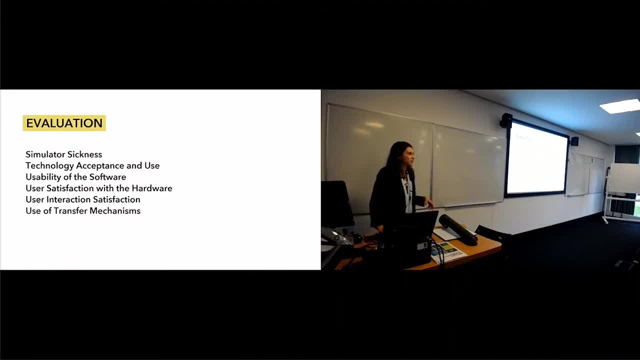 Because it's like the first thing. Oh, I don't want to use it because it will make me motion sick. Oh, I tried VR once and it's not working. But since each application is unique, environment is unique, You need to always think about how the person will behave in this environment. 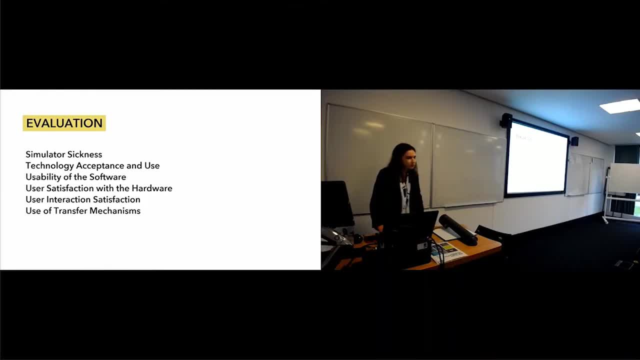 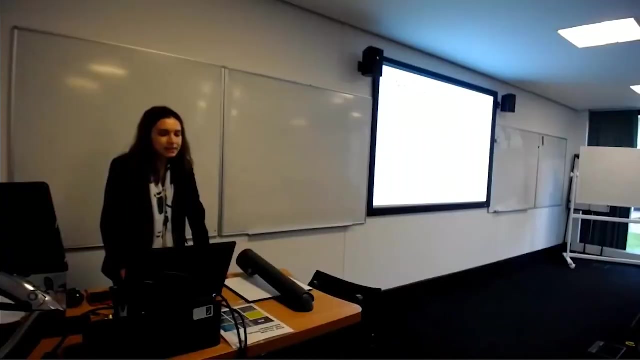 Simulated sickness questionnaire has 14 questions And asks you about your physical state and your physical experiences, Technology acceptance and use, Usability, user satisfaction, user interaction satisfaction And use of transfer mechanisms. Just in a second will be Technology acceptance is basically whether we want to use that technology. 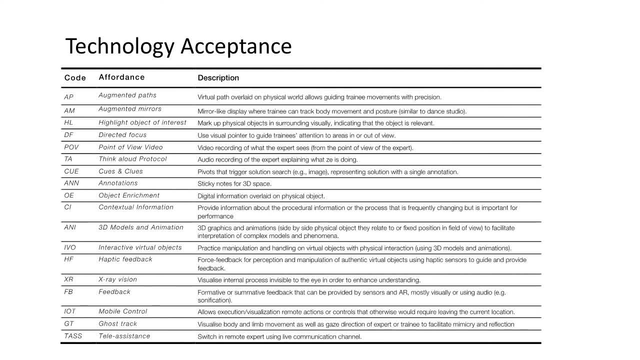 It's a method developed both for AR and classical technology As computer screens, website etc. And it tries to understand Whether people accept affordances of that system. If you recall the affordances topic from the previous lecture, Affordances are the means- physical or digital means- of the environment that we are using and perceiving from the world. 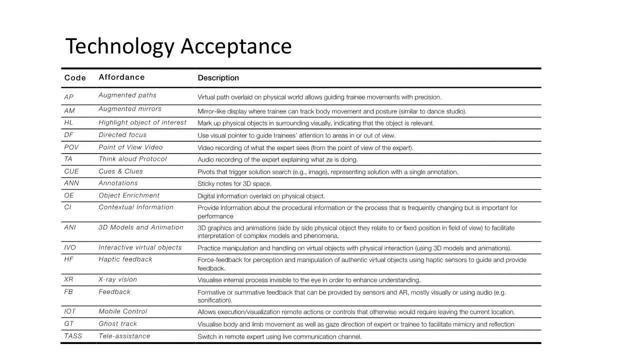 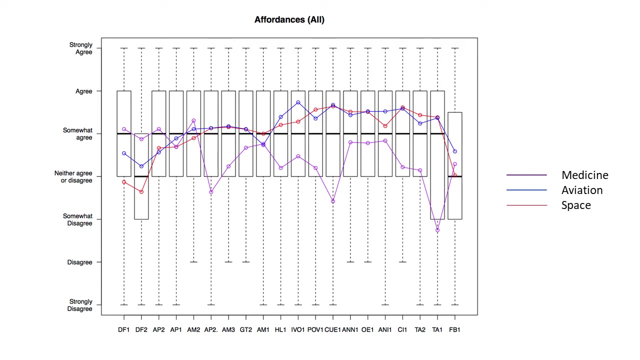 And technology acceptance. evaluate these affordances. For example, augmented path, directed focus, cues and clues: These are the ways system helps you to navigate and to walk through the application. So what are the sort of power that application gives you? For example, we- it's almost in March of this year. 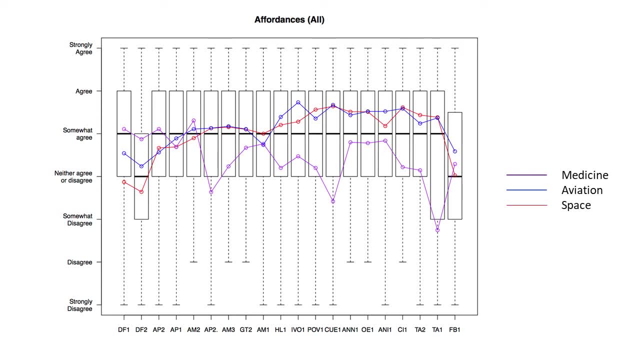 It's end of the three year project that we're working in the labs, Where variable experience for knowledge, intensive training And we were working within three different domains- Medicine, aviation and space. We run that technology acceptance questionnaire with them And we try to understand what is exactly missing. 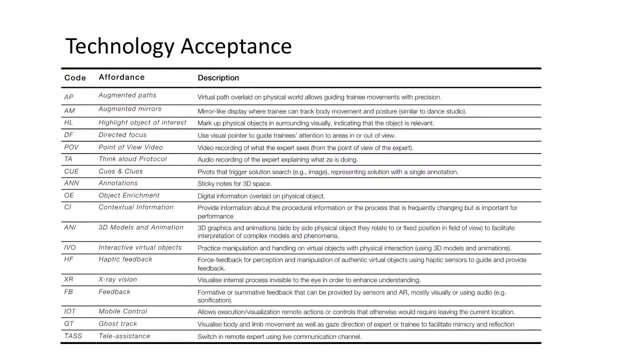 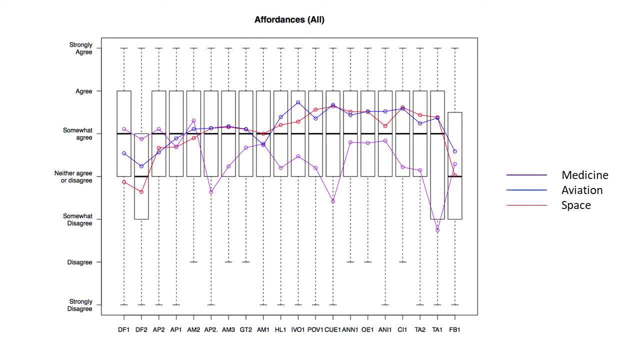 What we need to add to our system, Like feedback from the system Controllers or more 3D models and animations, And visually it really helps you to see your results And modify your system based on the user observations And answers and needs. 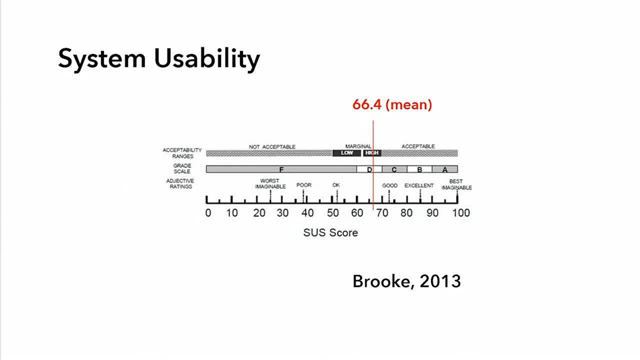 Also the classical method of the system innovation and system usability questionnaire. It's called SUS. It's a very standard way of evaluating usability. So in 2017, our system scored 66.4.. We're still analyzing the new data that we gathered during the last year and a half. 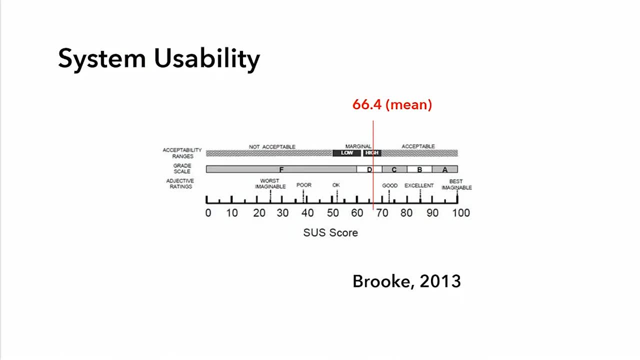 So I don't have, unfortunately, the new data, But you can see that it's pretty good. It's a marginal height, So it's above 50.. Good performance sort of, And this SUS questionnaire is also good, But I personally feel that system usability is something that needs to be added to other methods. 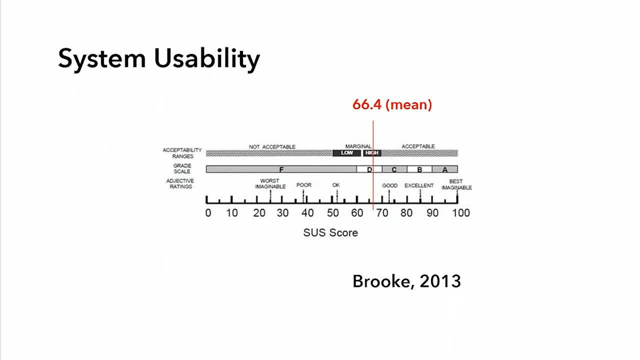 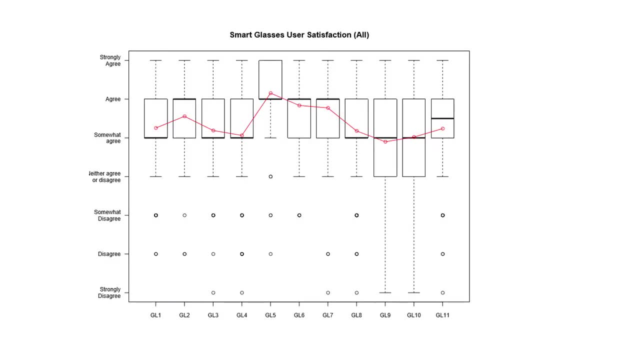 Like qualitative methods, for example interviews, or semi-structured interviews, When something is missing, from the point of spatial interaction, for example. There's also similar questions: Smart glasses, user satisfaction- That asks you less questions of whether you like the performance. 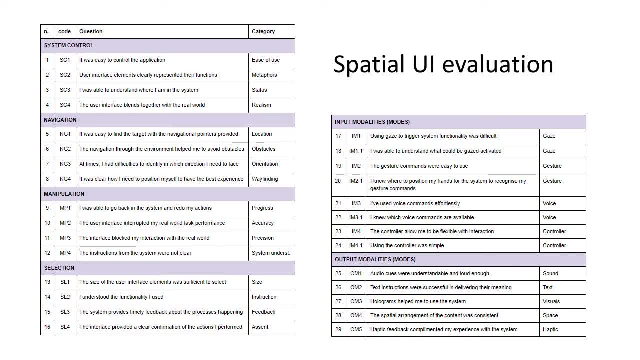 And the method we developed in the lab, in the performance augmentation lab here at Brooks, is a spatial UI evaluation. It's a set of 29 questions that are looking at the standard tasks that people perform in augmented reality: System control, navigation, manipulation, selection. 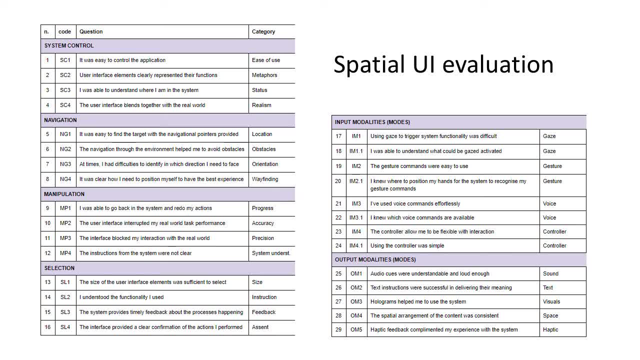 And different modes. So this is basically an advanced system usability scale, Because we found that system usability does not really reflect on something that spatial UI evaluation reflects, Like navigation in the environment and how people behave with the physical environment. So it's always about asking your question. 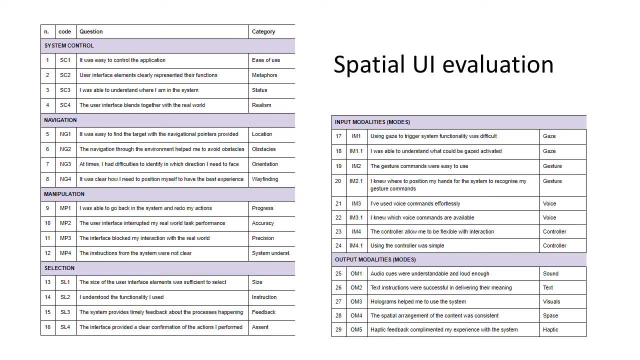 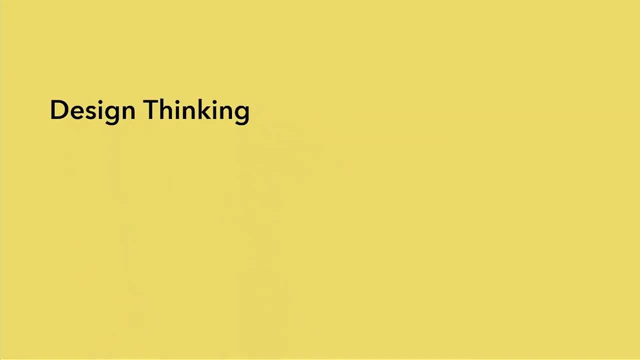 What is the aim, What I want to achieve, And by that you can choose the right and relative method. So I didn't have the right method, so we created a new one. We will start to work with the design thinking method. 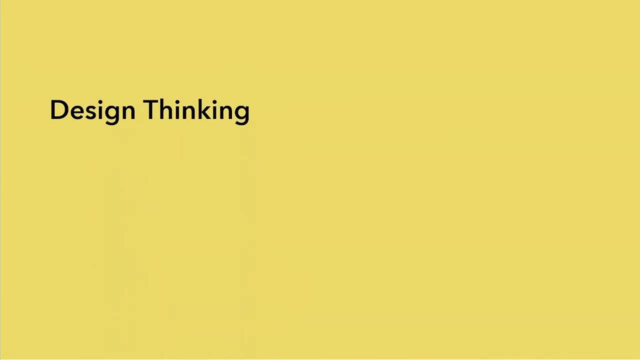 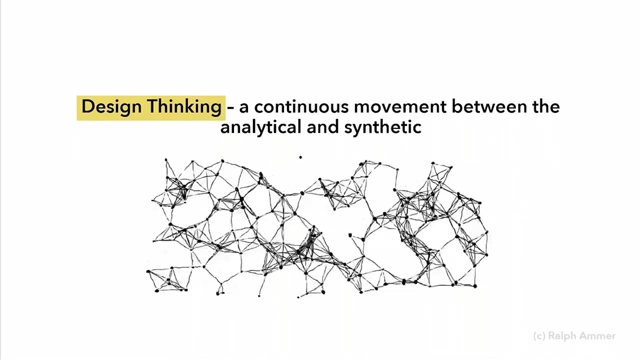 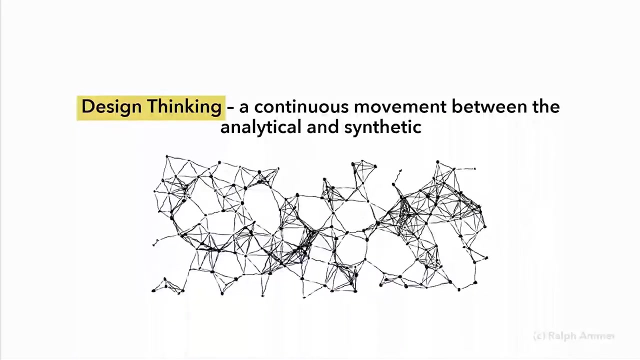 It's the classical HCI method that we will work during the tutorial. So basically, the design thinking is the continuous jump. it's like a loop between analysis and synthesis. So you create something and then you analyze it. You create your prototype And then you analyze it with the user. 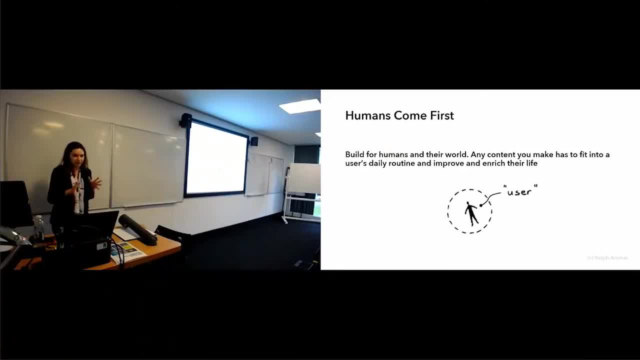 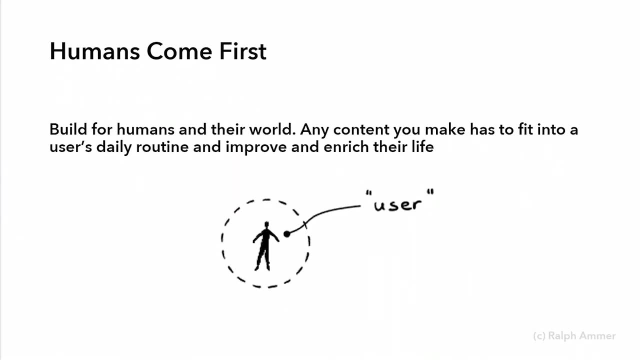 In design thinking, humans always come first, Because we build for them And I'm constantly saying that to you, that you need to talk to your user. Anything that you make has to fit their agenda, their everyday life, But not your imaginative world, unless you are designing for yourself. 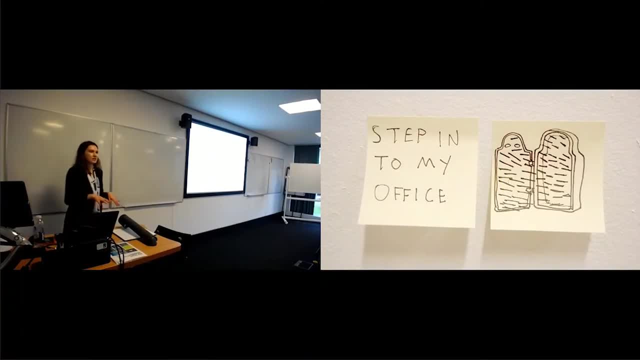 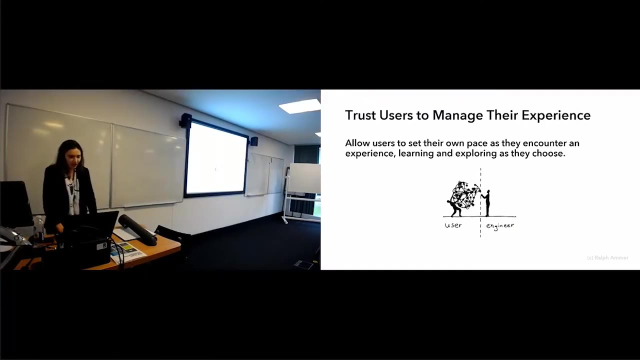 And it's about understanding them. It's about stepping into their shoes, It's about understanding their everyday life, Whether they are working in a factory, whether they are in the hospital. Even if it's painful, you need to do that. So, first of all, try to trust the user, to tell first things that you want them to tell. 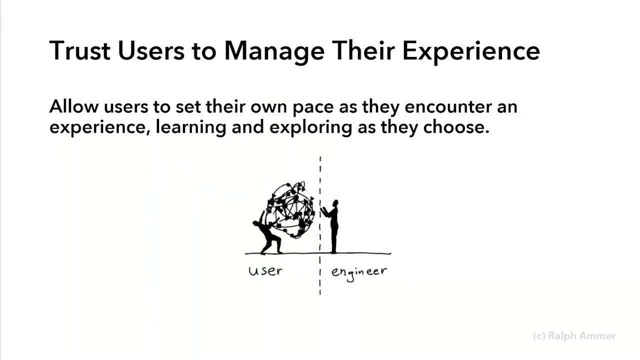 Allow the user to Express what they want, what they feel, Because they might feel pressured and not share that with you from the first point. So imagine that I think this graph is just perfect about. The user has all these preferences. I don't know what I want. 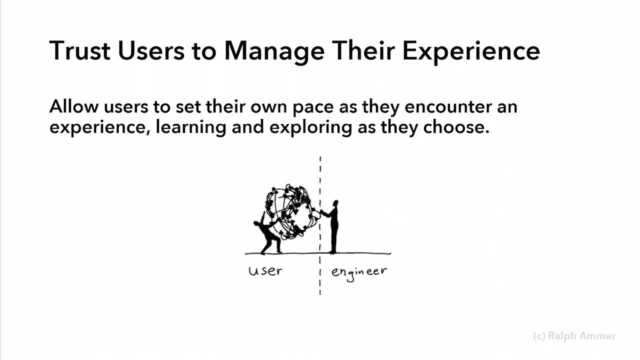 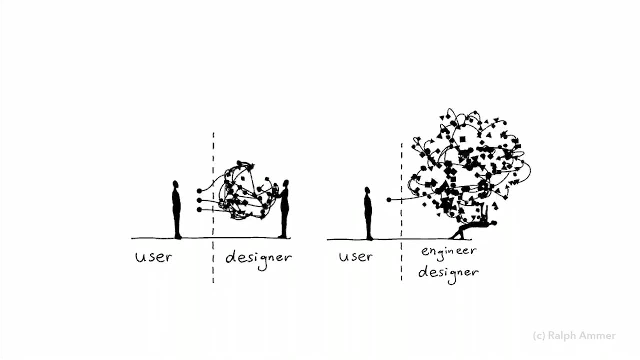 I'm always looking for something else. An engineer first tries to touch briefly the surface of the user, Tries to understand the scale of the problem. But It should be like this In reality: inputs and the system should be very, very simple. 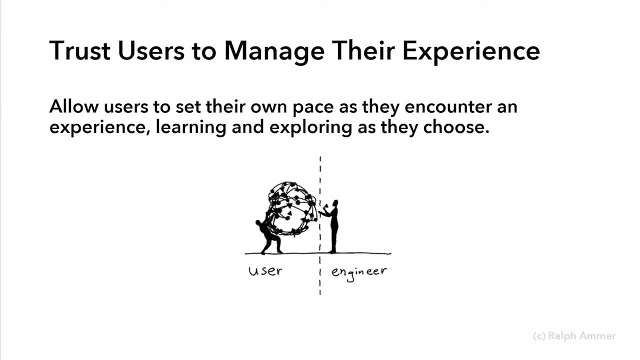 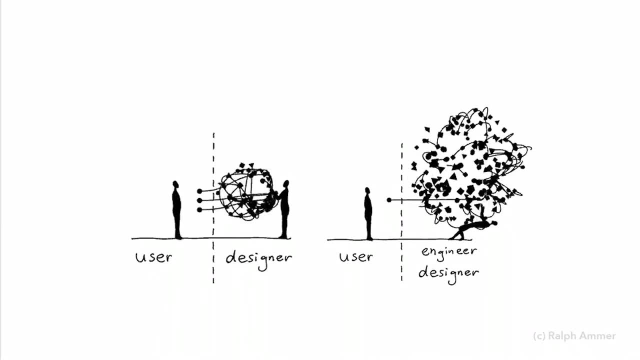 Not like this. It doesn't need to be coupled with all the things that you design. It needs to be really simple. You need to understand it, And this is a designer, an engineering designer. It's even more complicated, But the output is very simple and the interaction is very perfect at the end. 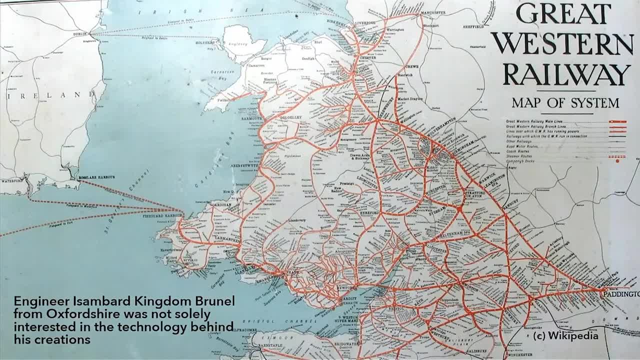 One of my favorite examples of implementation of design thinking method is the Great Western Railway Service in the United Kingdom. So many, many years ago there was an engineer from Oxfordshire, Isambard Brunel, And he was up to creating the railway service to connect London and Oxford. 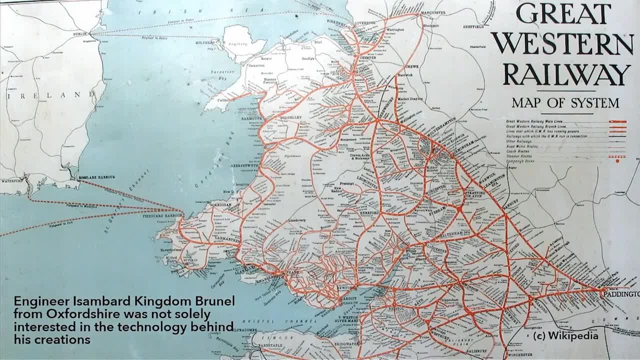 It was the first railroad And what he did. I think this is the first time someone tried to use the method of design thinking And he was trying to go from London, Paddington, to Oxford, to different other sites, And he thought, oh, it's really. 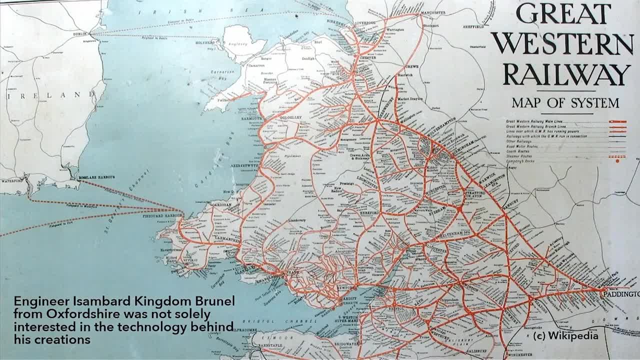 We can just go and build a straight line. Let's build a straight line and we will have our railway. But he thought, oh no, I want to have a perfect railway service. And what they did? They basically moved all the lands. 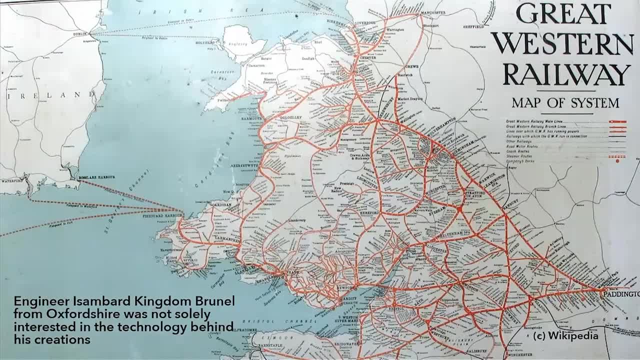 They removed the hills because they wanted to have the straight rail, So the user will have a nice and perfect journey without shaking carriages on the train, etc. So he really thought about how the person will feel using that train, About their everyday experiences. 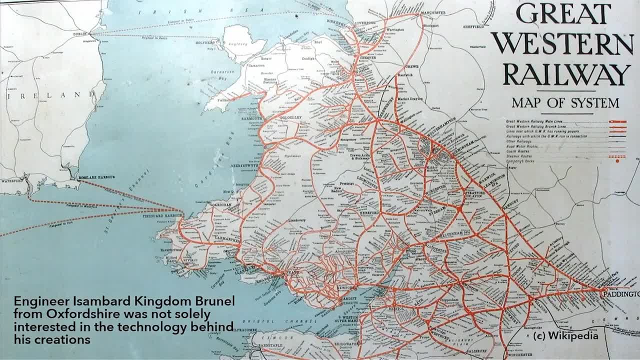 About the consequences of those everyday experiences On their lives and on the lives of others. So if you have a pleasant journey, you will be happy, satisfied. But I really love this example because it's also It's a national matter, So it's just one road. 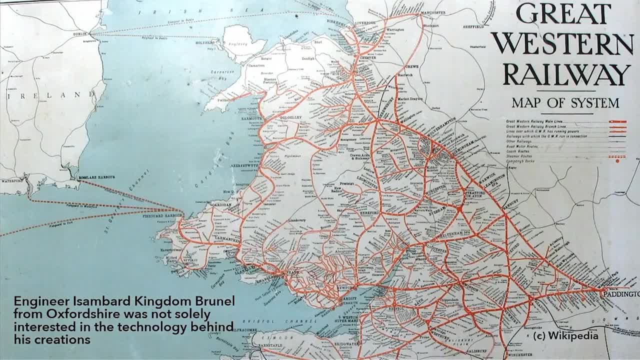 But it changed a lot of things in the UK. I know it's not so perfect actually, because I took a train from London this morning And it still was shaky. I was testing that- But it's better than if it were this hilly road. 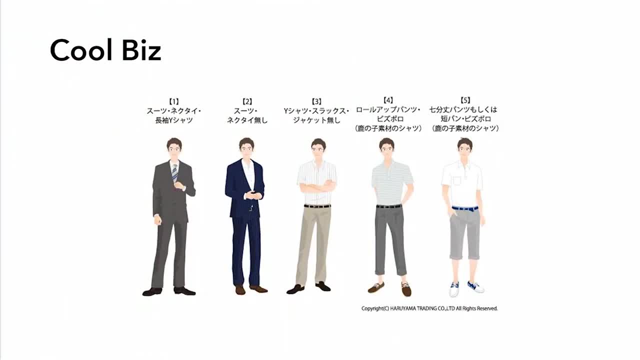 The second example I like is the Cool Bees campaign in Japan. They were trying to solve the national problem of raising levels of carbon And they needed to find a solution why it is happening. So the problem was that In the typical Japanese culture, you need to look very smart and presentable. 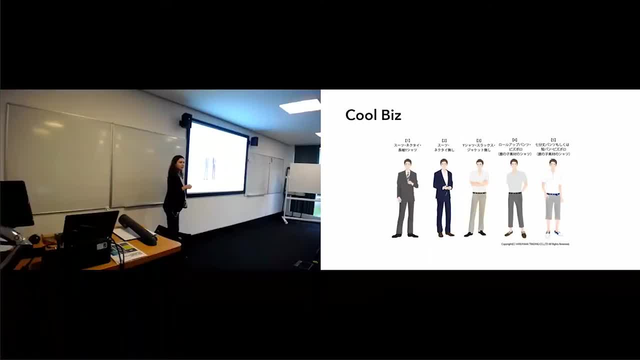 And in all offices they had air conditioning And air conditioning was set up to- let's pretend- 18 degrees And it was really absolutely okay for men to have a suit And they felt comfortable in that temperature, But for women, in 18 degrees they were freezing. 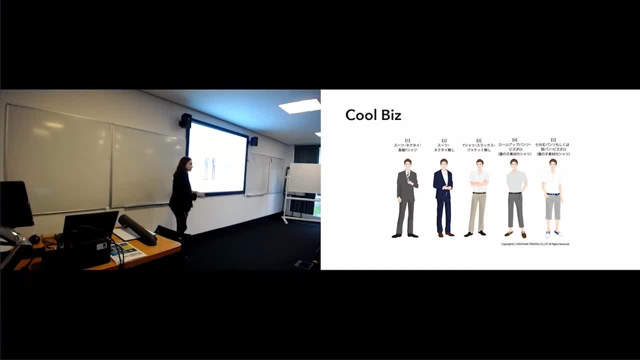 But they still needed to have the skirt and the short top. So they changed the level of carbon in Japan, I think 10 years ago, by changing the rules of the everyday uniform. So they reduced the temperature of air conditioner to 20.. 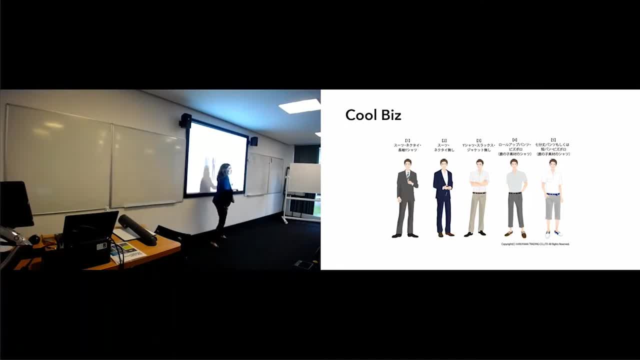 And they still were able to feel comfortable in that temperature, but without feeling ashamed. They were ashamed of how they feel because the prime minister and all the government in Japan, they highly supported this campaign. They had the special fashion shows that this is okay in Japan to have casual look. 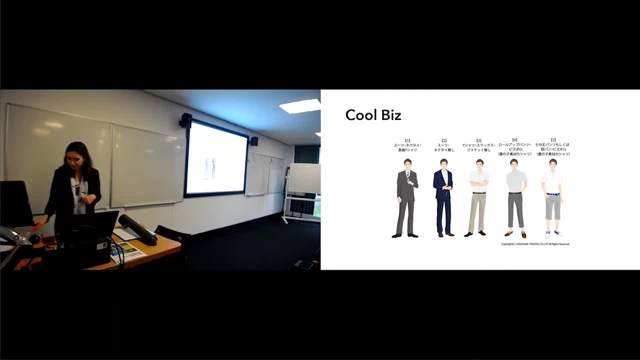 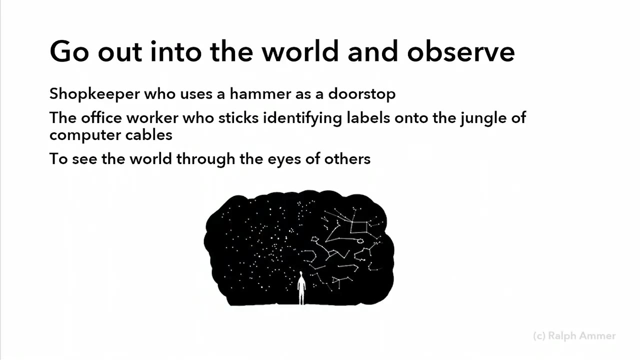 And they saved the country from ecological disaster by just changing the perception of how it's okay to look in Japan. Design thinking encourages you to observe and see some hidden path that you might not see from the first time. Sometimes it's really a hidden journey. 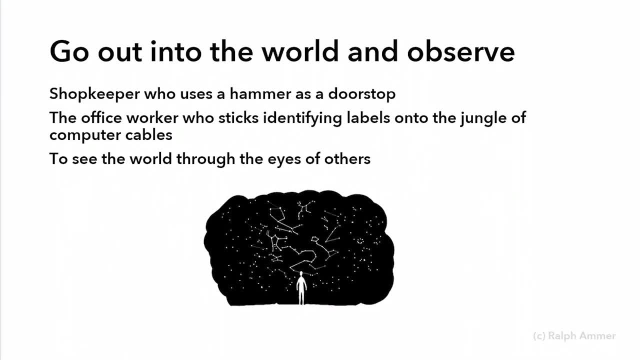 My personal discovery is that in Norway people don't like to look up. Why people don't like to look up? Because we had this application in the yard with all the navigational systems And they didn't really look at the top part of the experience. 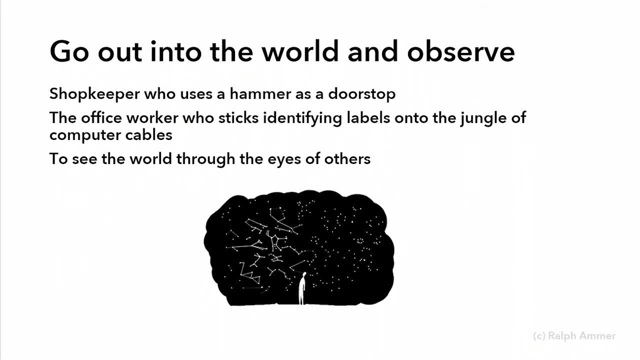 And I tried to talk to them outside of the office hours, Like why do you like things on top of the application, Why don't you just look there? And it was absolutely like no reasonable answers, Like I don't know, It's just this happens. 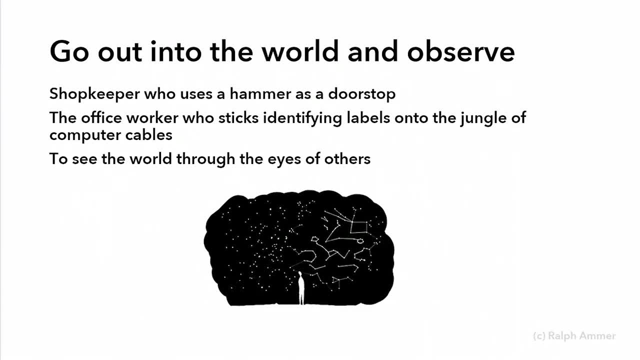 We are just so focused on things on the sides And then at the end of the day at some point I noticed that Norwegians especially above the polar circle. it's really cold there, It's freezing. Sometimes it's like polar night for the half year. 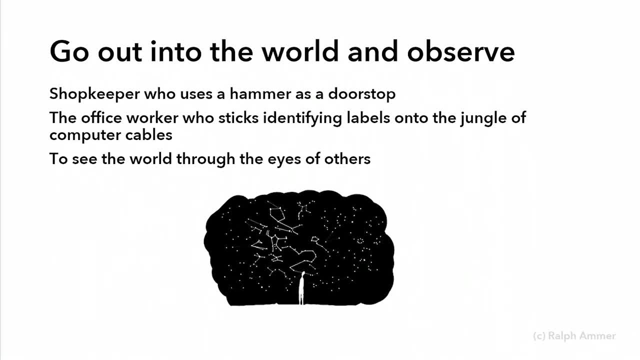 And they commute in the underground tunnels And tunnels. they have really bright lights on top of the tunnels So it's really painful for them to look up. That's why they feel uncomfortable looking up. Sometimes discoveries they just appear through random conversations. 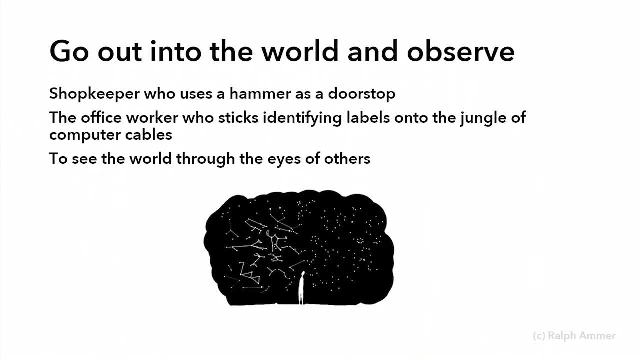 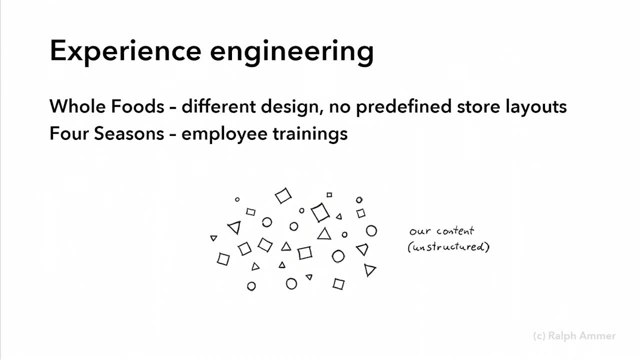 But try to look at the world through the eyes of others, Because sometimes it's really unexpected and unimaginable discovery. Another two examples of experience: engineering: Do you know who? Whole Foods supermarket. So each supermarket has its own different design. So each Whole Foods in the world is different. 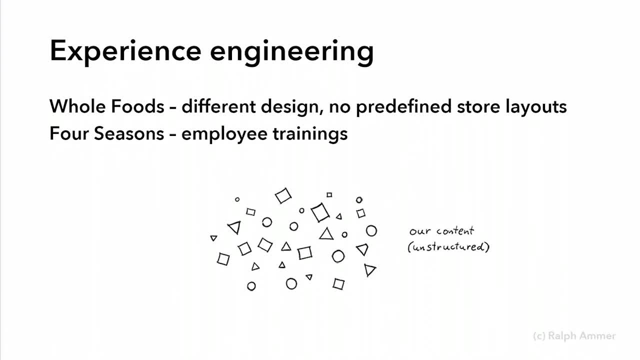 There are no predefined store layouts at all, Because they just want to create a customized experience from each city And, for example, the hotel Four Seasons. they do employee trainings And for each employee to perform perfectly, they arrange a one-week stay at this hotel as a user. 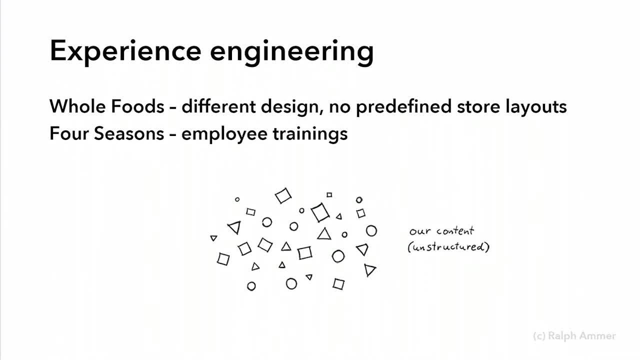 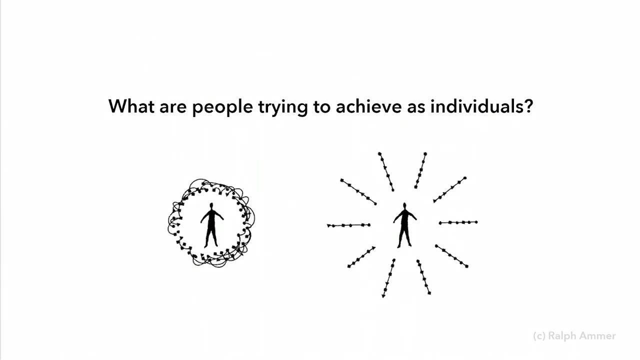 as a person who is on holiday And they observe what type of service they're supposed to receive And during their work they sort of follow that personal example. So also ask your questions: What are people trying to achieve as individuals in your experience? 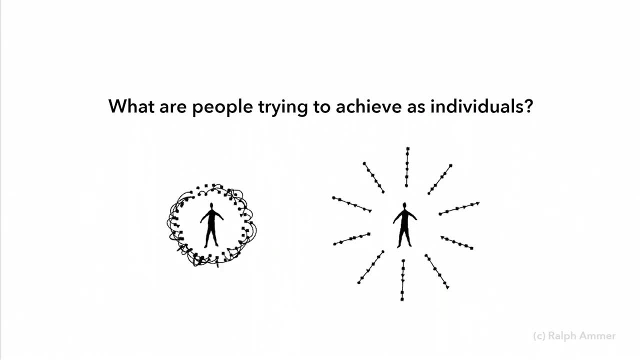 What is the aim of this application? Do they want to be healthier, fitter, smarter or happier, Or they just want to know more about a particular thing? Or you just want to help them to solve the problem of daily commute? I don't know. 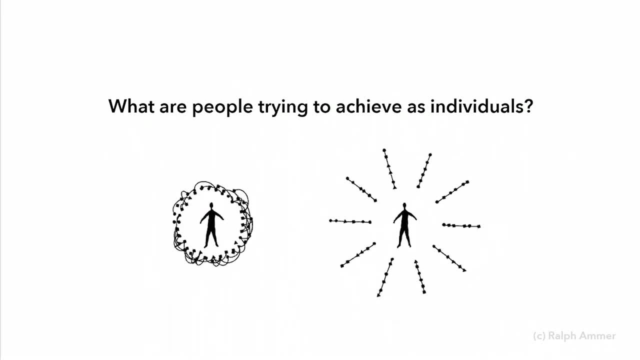 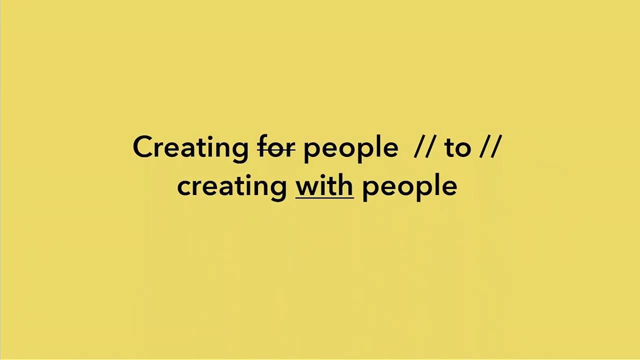 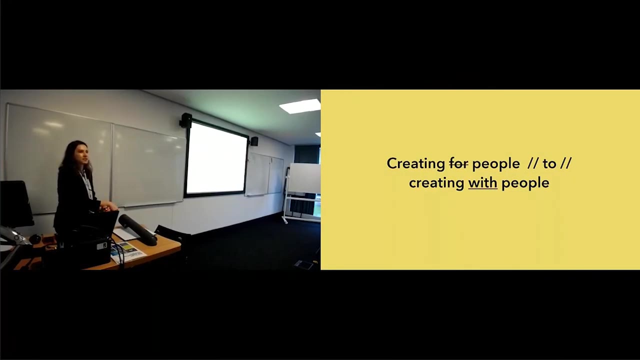 They don't know what to listen in the evening, Or they're struggling to learn anatomy or something else, And in this case you're creating not for people, but you're creating with people, because only with them you're able to find discoveries. 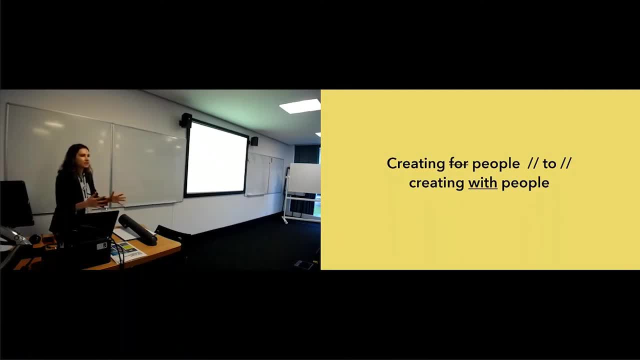 Maybe next week you will think, OK, I have this idea, I want to do this, Like straight away, I need to do this. But maybe your idea is just for yourself. It's just an idea for one person. You need to talk to people who had this problem. 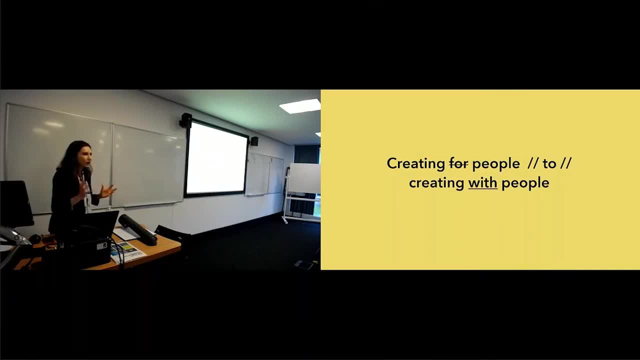 or had experienced something. Maybe you can recall someone complaining about something And you need to keep that context in mind, Keep context of the conversation involved. Will people use your system at home or somewhere else, Or they will use it once per week? 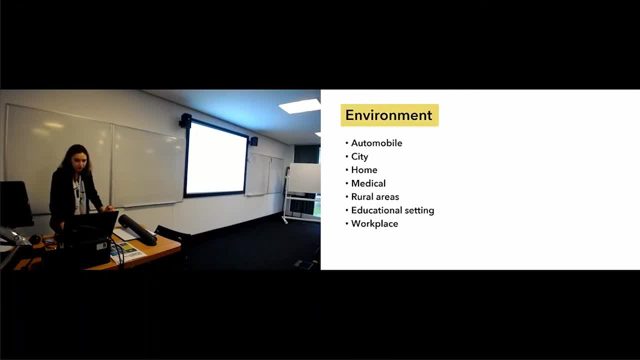 Every week you need to think about the environment, like city, home, medical, educational setting, workplace, because your design will be predetermined by this environment And you will use different research methods for that as well.